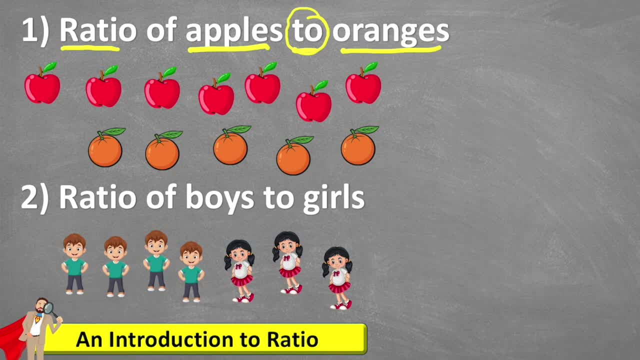 Our first one. we're going to simply just count our apples and we've got 1, 2, 3, 4, 5, 6, 7.. So we have 7 apples. to how many oranges? 1,, 2, 3.. 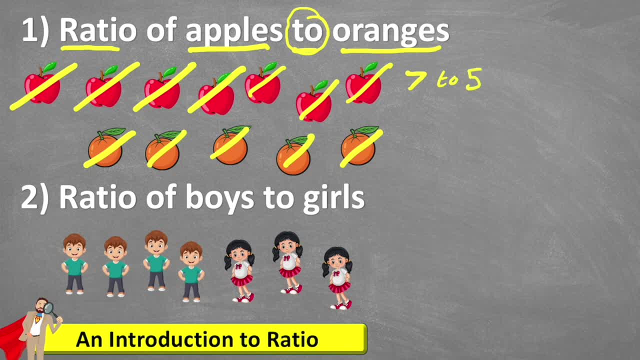 4, 5.. So we have 7 to 5.. So our ratio is 7 apples to 5 oranges. That's the first way of showing it. Then we could show it using the colon, which is the symbol for ratio. 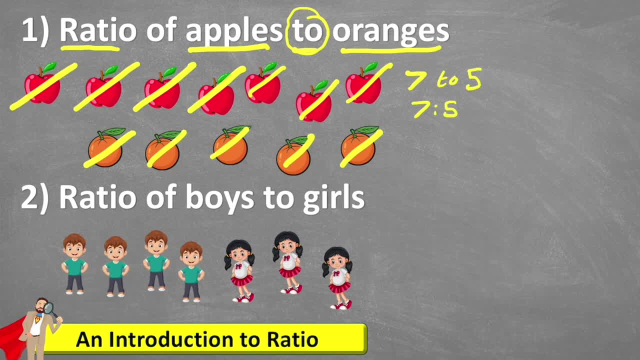 So we could show 7, colon 5.. That's another way of showing it, That's the most common way of showing it. But then we could also show it in a fraction, because ratios and fractions are very closely linked. So we could also show it with being 7.. 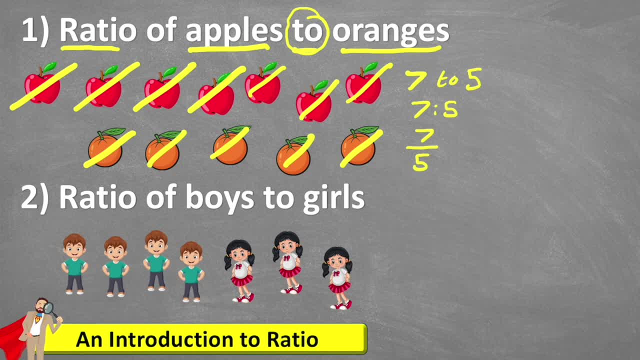 So we could show it with being 7 over 5. We have 7 apples to every 5 oranges. OK, so let's have a look at this second example. This one says the ratio of boys to girls. So again, I'm going to look at the 3 different ways that I can show this. 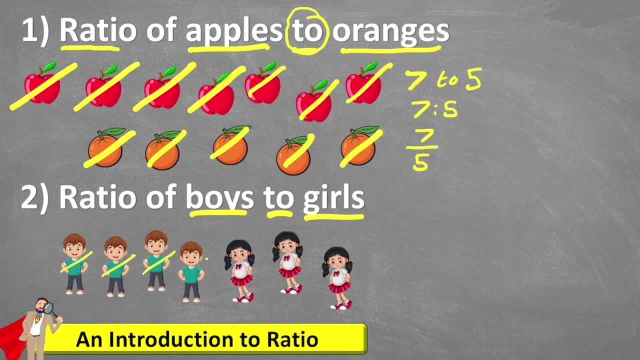 And I can see that I have 1,, 2,, 3,, 4 boys. So I have 4 to how many girls? 1,, 2,, 3.. So I could show it 4 to 3, or I could put 4, colon 3.. 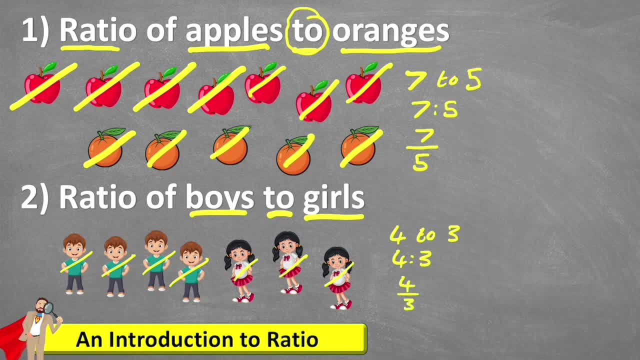 Or I could put 4 colon 3.. Or I could write 4 over 3.. But at this point I'd like to just show you something. Now, if I get rid of one of these girls boom, just like that. 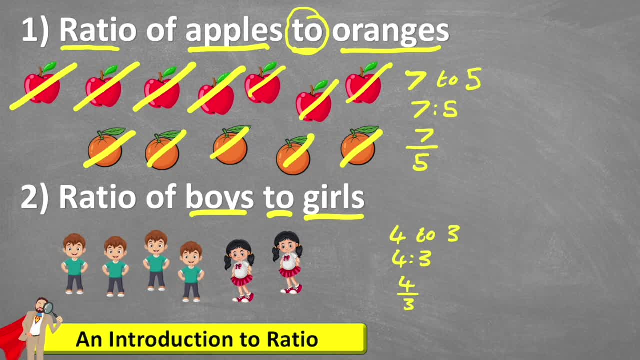 Now we have a totally different ratio. Now, of course, we have 4 to 2.. 4, 2, or 4 over 2.. But what we can actually see is that we can simplify this ratio very much, in the same way as simplifying a fraction. 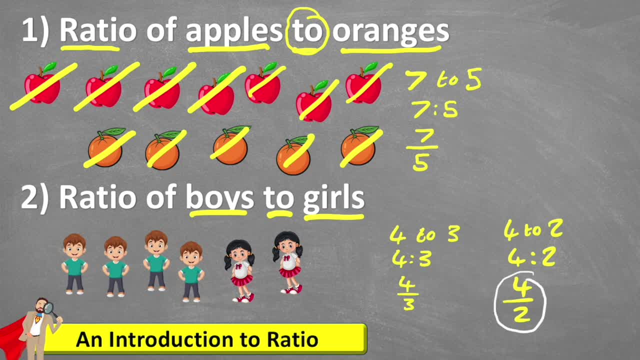 And if we were to look at this fraction, this 4 over 2, we might be able to see that actually, this just shows that for every 4, I have 2 girls. So for every 4 boys I have 2 girls. 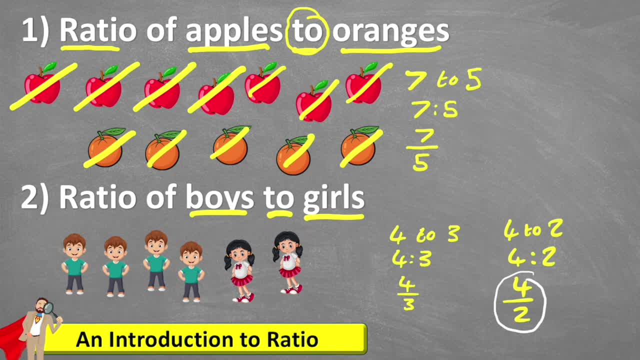 But what we might also be able to see is that we have for every 2 boys we have 1 girl, And again for this second group, every 2 boys I have 1 girl. So my simplified ratio could be 2 girls. 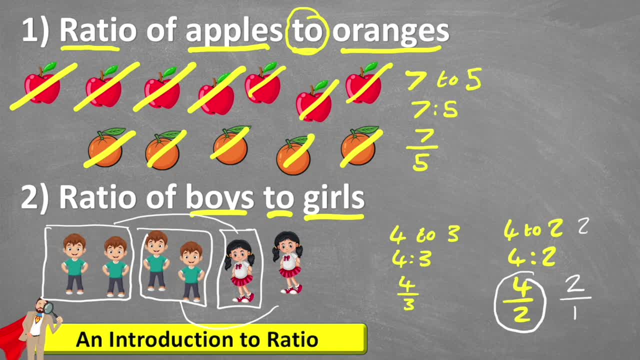 2 over 1.. And again, I could show that with 2 to 1 or 2 to 1.. Just like that, And this would be the simplified version of the ratio, And just like fractions, we always want to show the ratio in its simplest form. 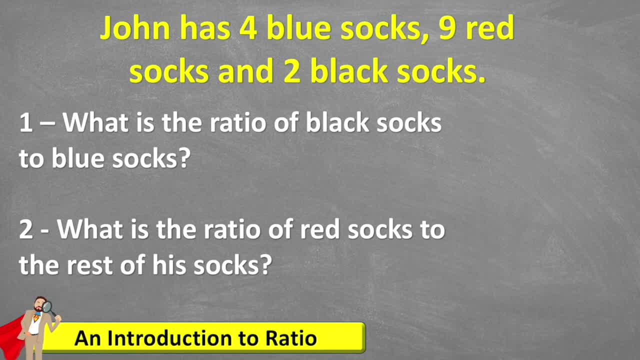 Okay, let's have a look at a word problem then. This says: John has 4 blue socks, 9 red socks and 2 black socks. First question says: what is the ratio of black socks to blue socks? So it's asking you for black socks. 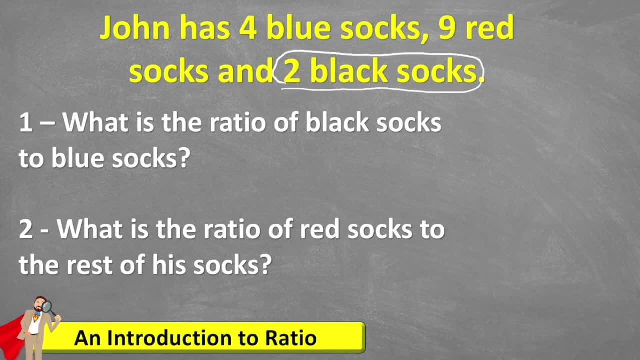 So let's put a line underneath the black socks to blue socks And we have 4 blue socks. So I've got to be very careful and follow what the question said And it said the amount of black socks to blue socks. So I have 2 black socks to every 4 blue socks. 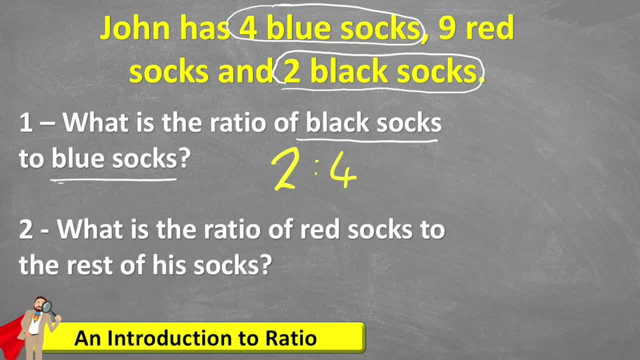 So my ratio is 2 to 4.. Now what you might see is, if we make this into our fraction 2 to 4, you might see that this can actually be simplified. I can divide by 2 and I can divide by 2.. 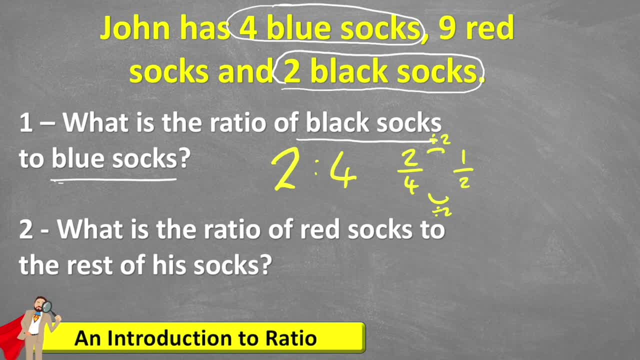 I'd get 1 over 2.. So my ratio is actually 1 to 2.. Then my second question says: what is the ratio of red socks to the rest of the socks? So this is a two-step problem. So how many red socks do we have? first of all, 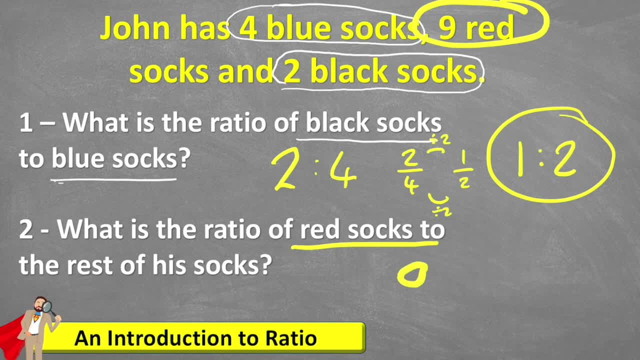 Well, I have 9 red socks, So I know that I'm going to be starting with 9 to something. And then I need to actually calculate my blue socks and my black socks, And 2 to 4 is 6.. So my ratio is 9 to 6.. 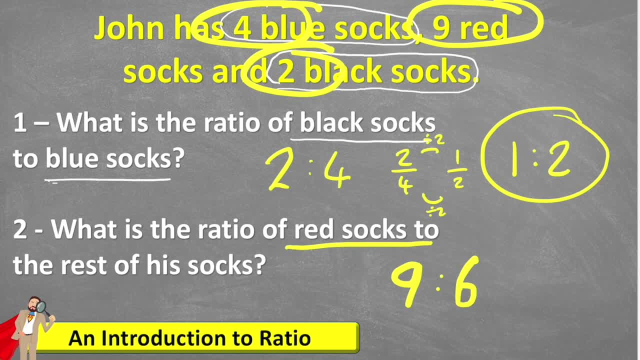 But again, I think I can simplify this And just following the rules of simplifying, whatever I do to one number I must do to the other And I have to use multiplication or division If you're not too confident on simplifying fractions or simplifying in general.